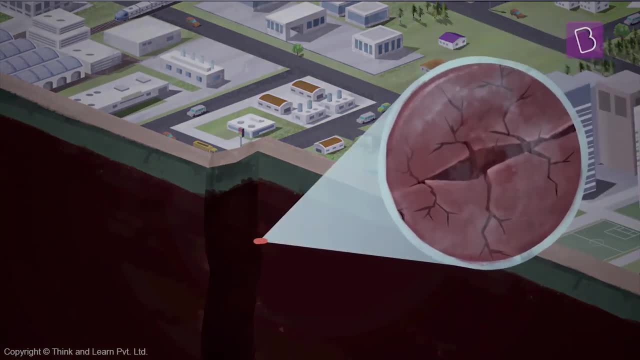 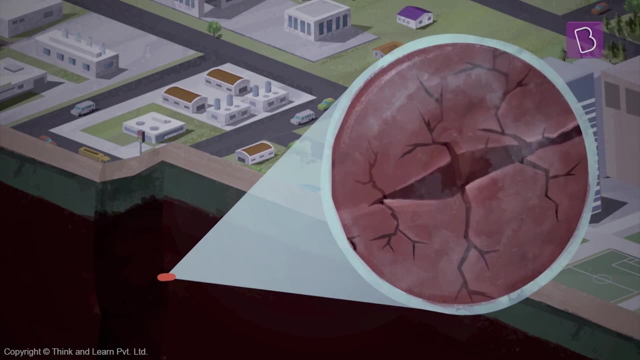 This is because these plates have several irregularities on them. When these plates slide past each other, the jagged edges of the plates sometimes get caught against each other. When they get released, our plates will slide past each other. After this tug-of-war of tectonic plates, the energy released causes vibrations. 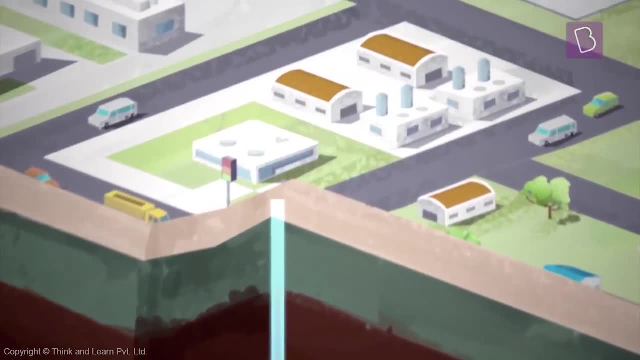 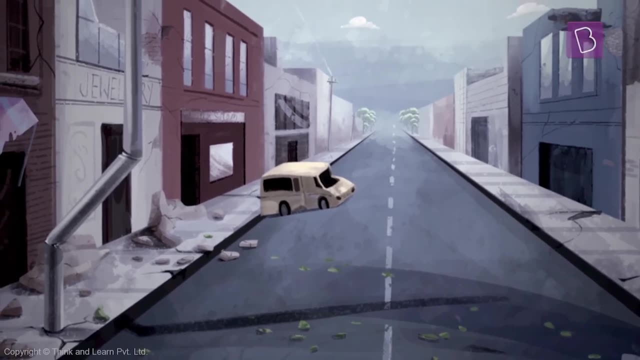 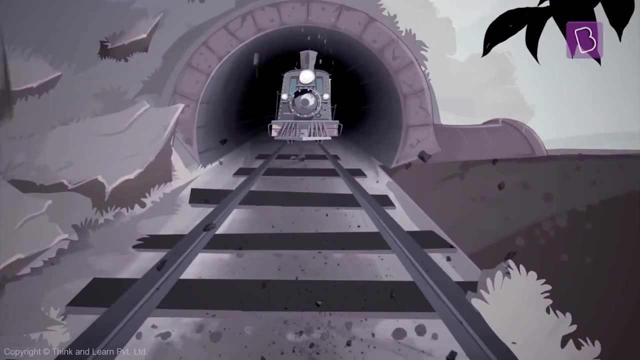 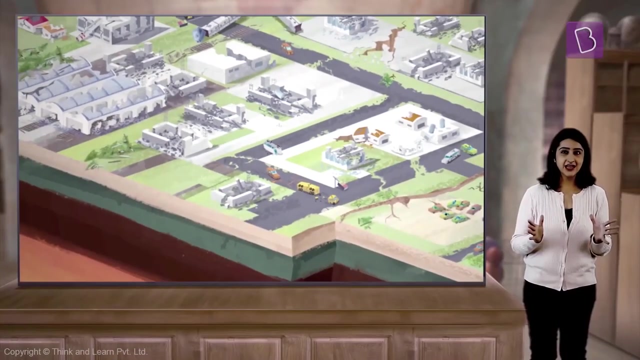 These vibrations move in the form of waves and shake the earth violently. This violent shaking is sometimes so intense that it can collapse entire buildings and cause huge dents on roads. They can even turn railway tracks and cause shifts in certain landscapes. Sounds scary, doesn't it? 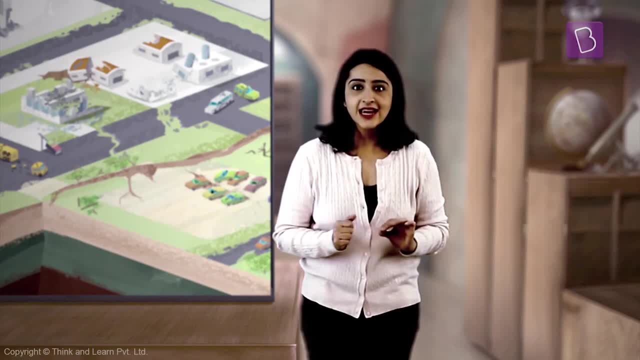 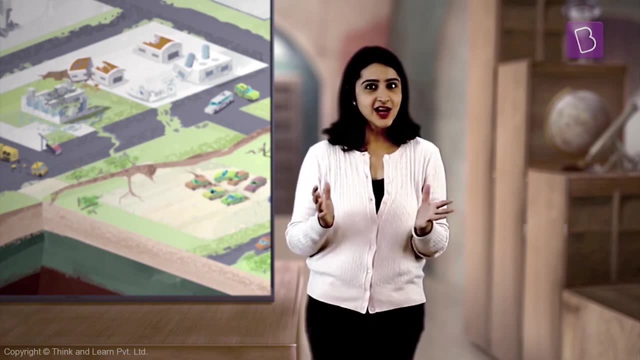 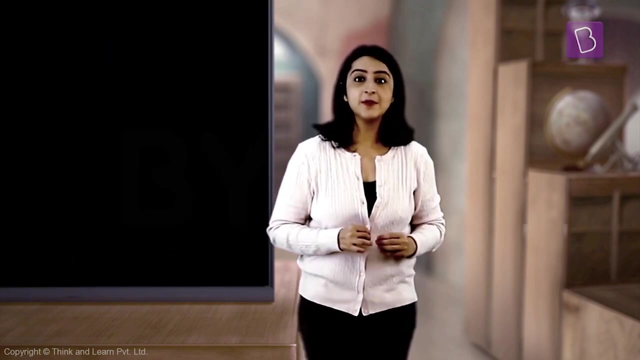 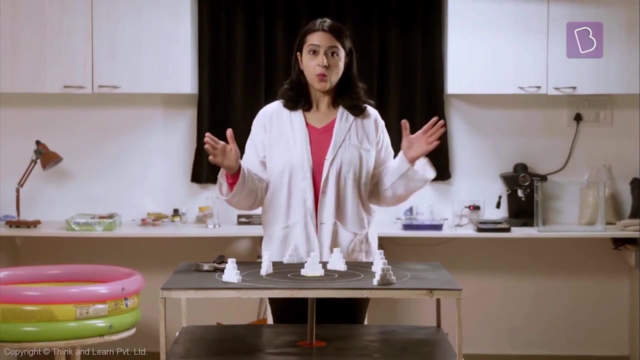 But think about it. How does the shaking under the surface of the earth destroy so much above the earth? Isn't it strange? Alright, let's use a demonstration to understand how vibrations under the surface cause havoc on the surface. As you can see, we have created a wave. 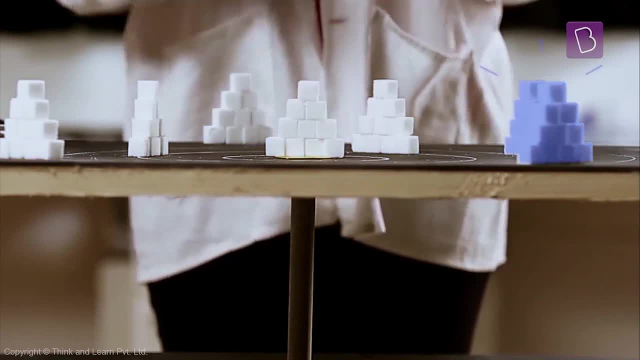 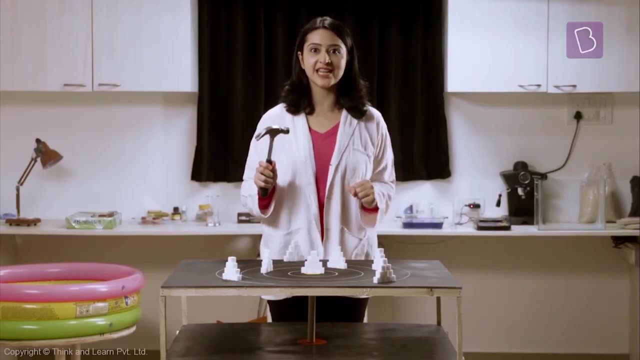 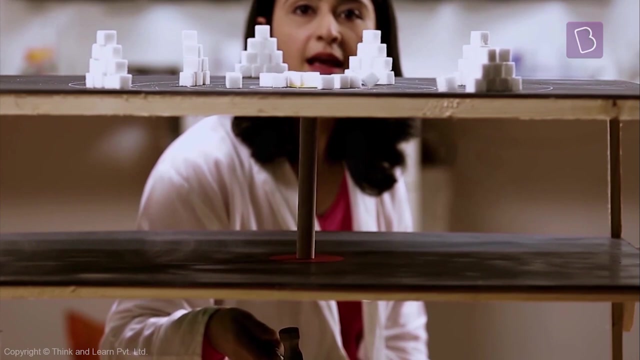 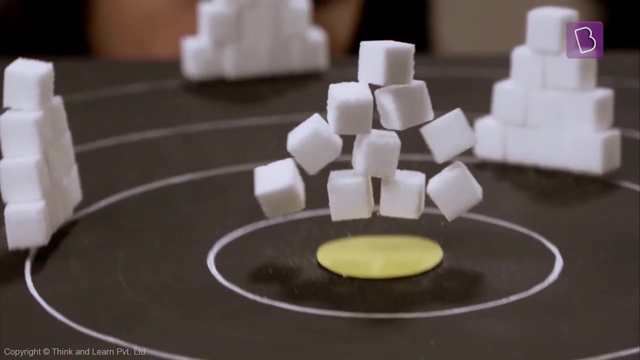 As you can see, we have created a wave. We have created structures with sugar cubes here. What we are going to do is create an artificial earthquake with a hammer from under this table. You see that The sugar cubes near the centre fall first, because they are vibrating the most. 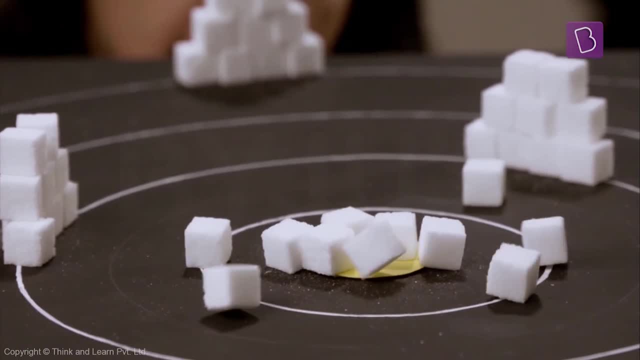 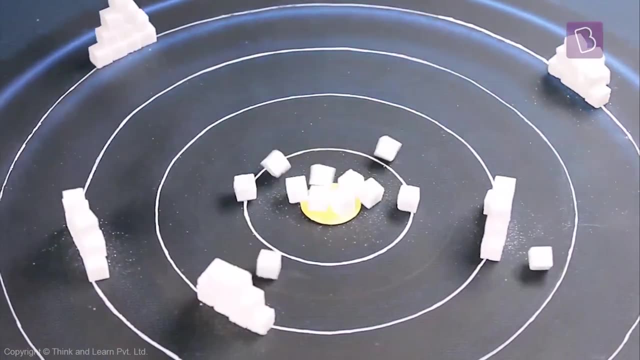 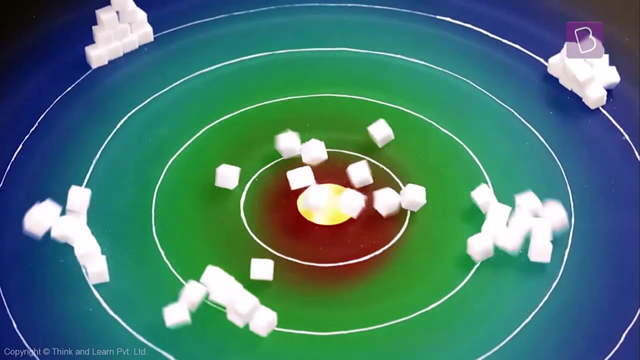 And then they gradually decrease in intensity. and then they gradually decrease in intensity. Why is that? This is because, when the vibrations are created, they travel as waves, which are the strongest at the place where they originate. They gradually reduce in intensity as we go further from the centre. 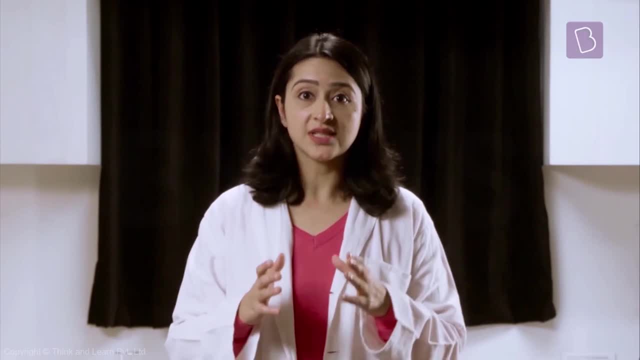 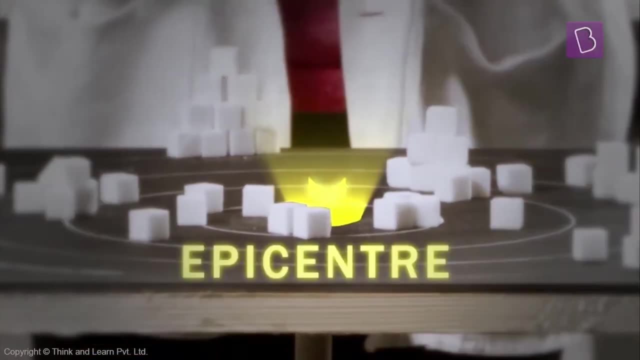 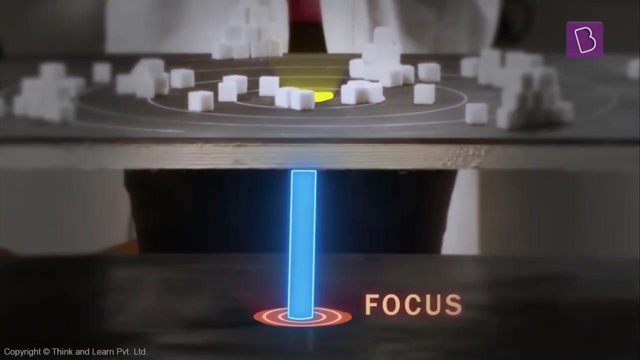 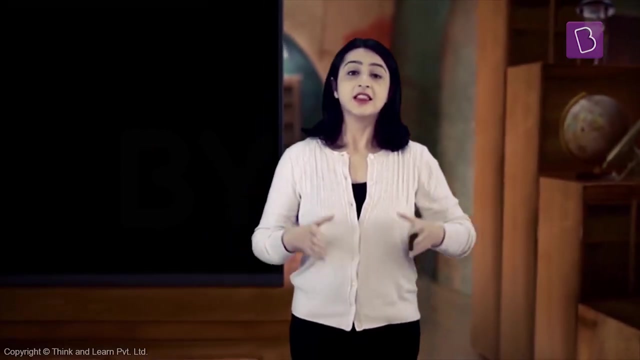 When it comes to the earthquake, the place on the surface where the earthquake seems to fall be originating from is called the epicenter. The point inside the earth right under the epicenter is called the focus. In our demonstration, the common center of all these circles is the.